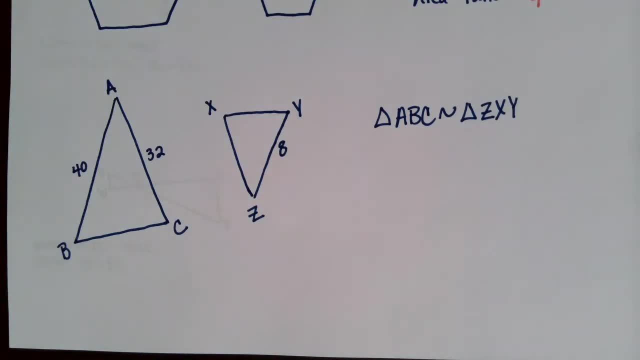 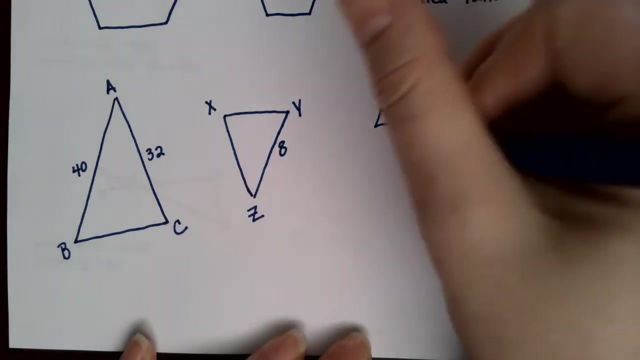 For learning to get 5.2.3,. you are going to be given similar polygons, similar triangles and asked to find a missing value, And so why don't you pause the video and get this problem drawn the best that you can? And now, once you have this drawn, we are going to find 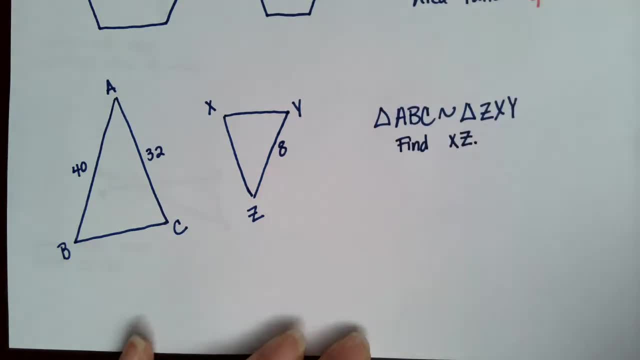 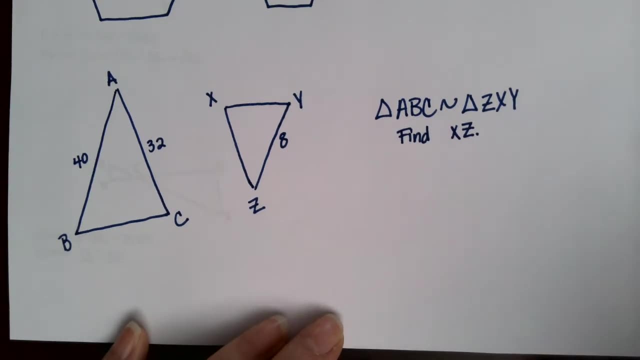 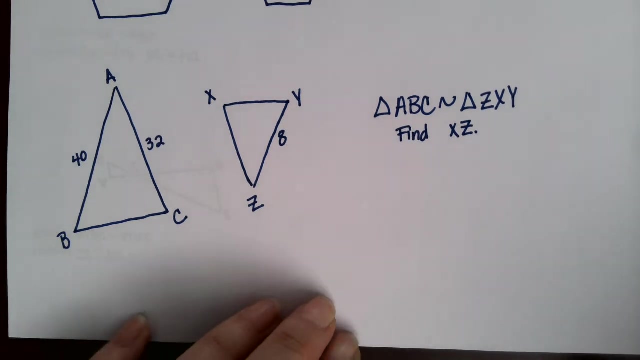 side x, z. So that's going to be our value- that we are missing, And so for this, you want to set up a proportion and include the side that you are missing. So I like to just start with the side that I'm missing, And so that's going to be like my top shape is the. 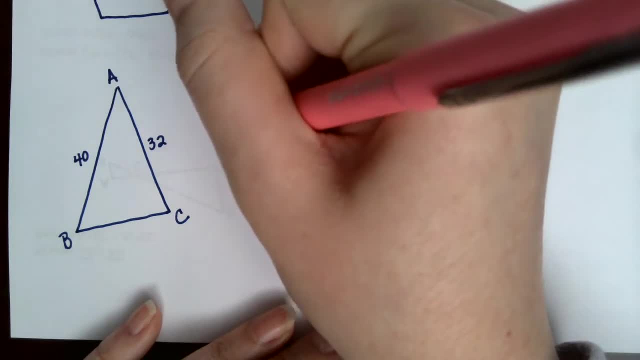 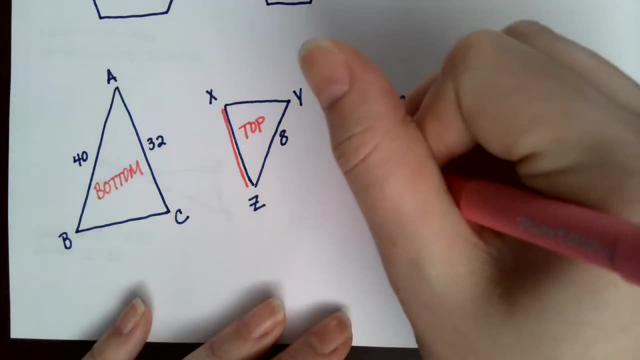 one where I'm missing. So this side is what I'm looking for, And then my bottom shape will be the other one, And then my bottom shape will be the other one, And then my bottom shape will be the other one, And I always start with that missing value. So when I set up my proportion, I'm going 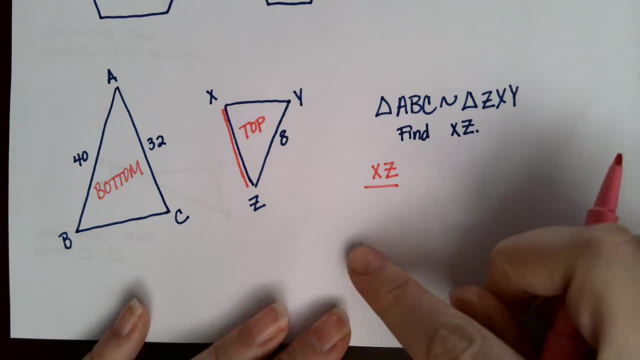 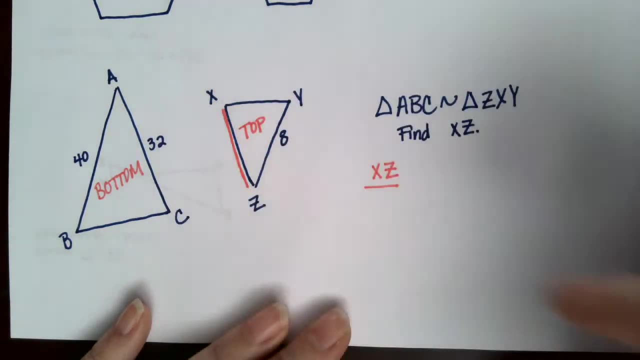 to start with x, z, And then, when you set these up, do not use your picture. The pictures can be misleading. You don't know if this was just flipped upside down or if it was flipped and rotated. And so we want to use our best friend, We want to use our similarity statement to find: 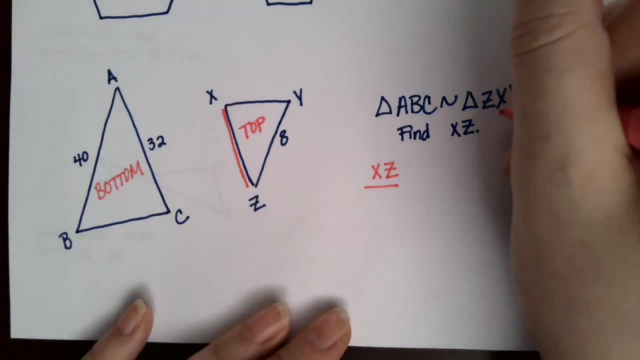 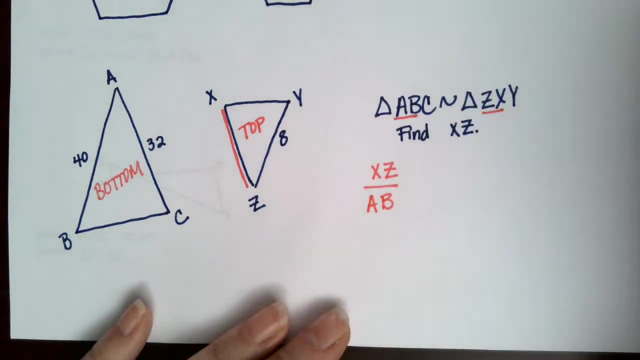 our corresponding sides. So x- z are the first two letters And a- b are the first two letters. So this corresponds. Now we need to set up another proportion over here, And that one needs to be so. here's our top shape, And it needs to be a value that we're. 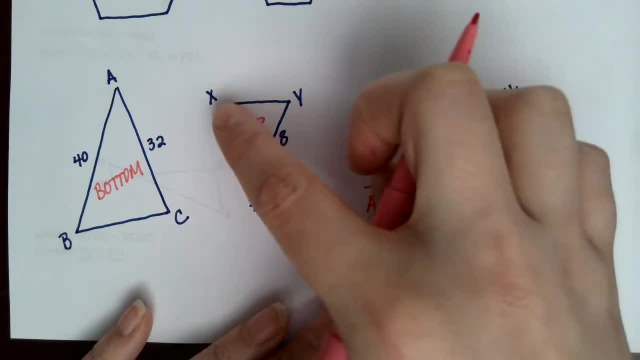 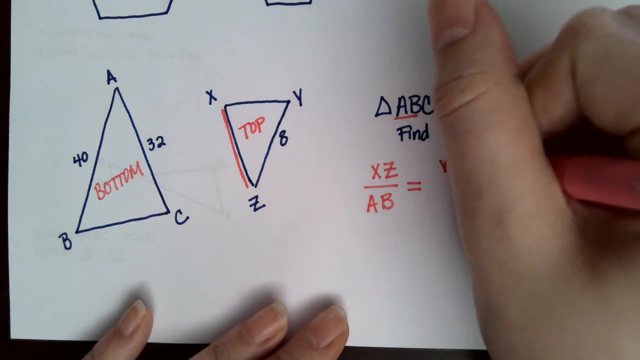 given the side length. So my only choice is y- z. I can't use this because I don't know this side length. I need to have a known value. So I'm going to start with y- z on top over here. 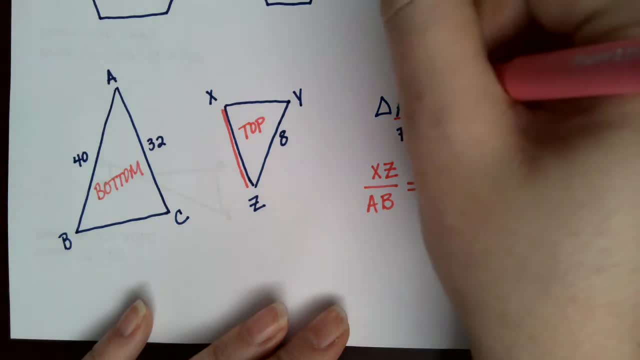 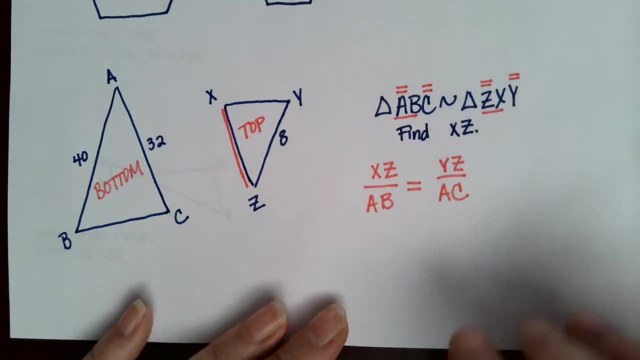 And then I'm going to set up my proportion over here, And then I'm going to set up my proportion over here, And then y, z are our first and last letters, And so that's going to be a, c to correspond. So again, we want to use our best friend to set this up, not the picture. 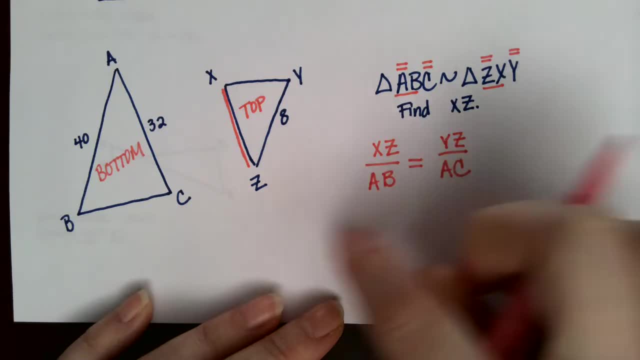 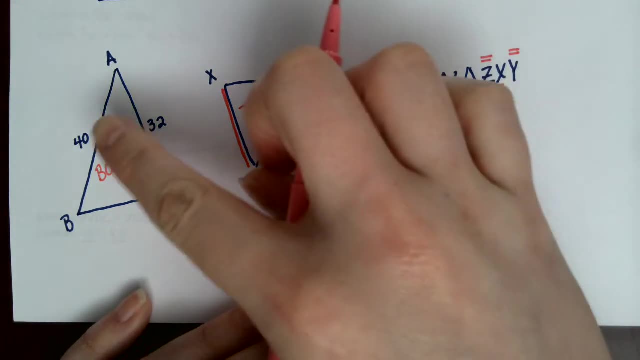 Once you take your time and set up this proportion, you just got to plug in the values that you see. So x, z is the one that I'm missing, So I'm just going to leave that as x, z, a, b is 40..